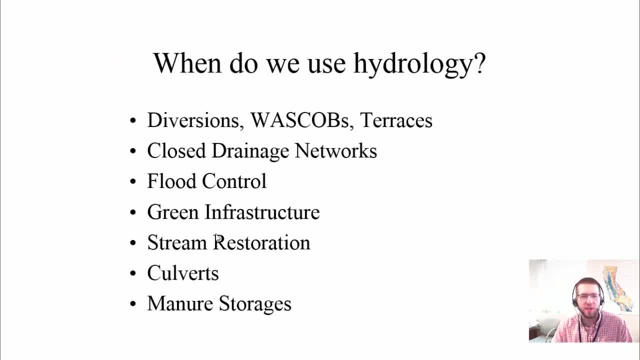 Now what are some of the BMPs that need hydrology studies? We've got diversions, WASCOBs, terraces- These are all agricultural practices. Closed drainage networks are typically in urban areas. Flood control can be both. Green infrastructure practices are typically urban again. 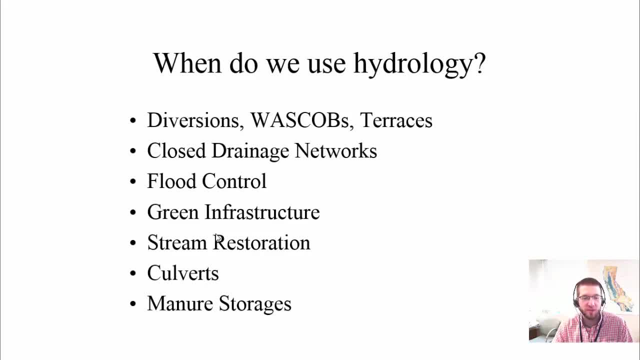 Stream restoration is typically rural Culverts, manure storages, And the thing I want to highlight is that some of these practices only require peak flow rates and others require you to know the entire storm volume. So a peak flow rate is achievable, say using EFH2 or the rational method. 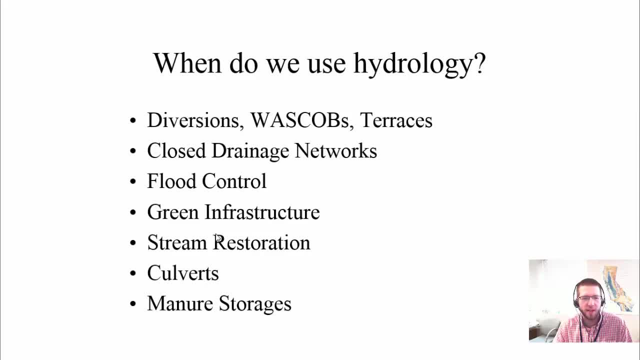 But in order to get the whole storm volume, you'll need something more complicated. So that's just something to keep in mind. If you need the whole storm volume, you'll have to develop a hydrograph and use a method that provides that. 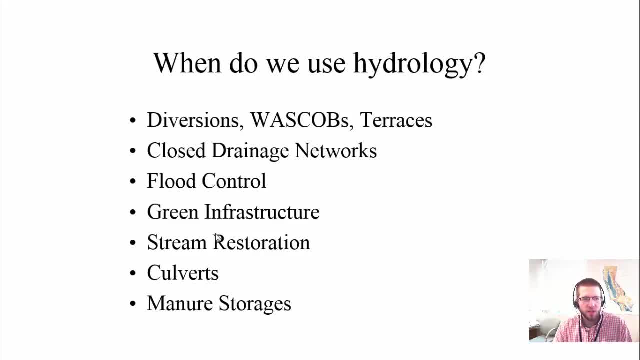 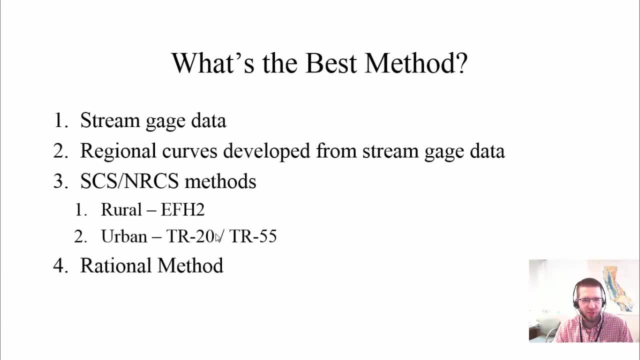 And we'll cover what a hydrograph is in a moment. So, first off, I want to give you a sense of what is the best method of hydrology. You know how we're coming up with stream flows or storm volumes. What's the best method? The best method is stream gauge data. 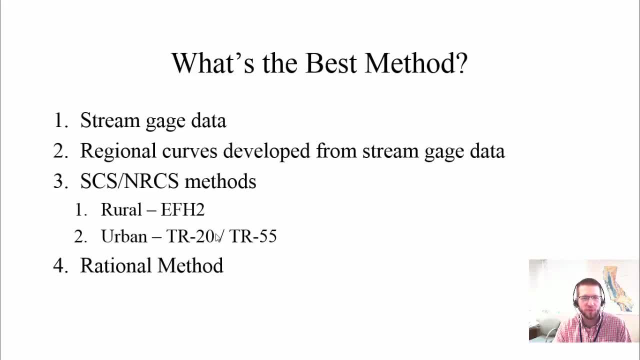 OK, this is an actual historical record of storm flows at a site. OK, obviously the problem is stream gauge data only exists for streams of a certain size And most of our hydrology studies are for small watersheds. So it's rare to find a stream gauge near your site, unless you're doing a bridge opening or something. 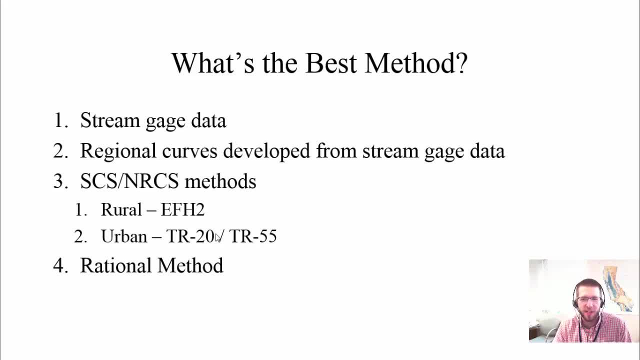 OK, the next best option is regional curves developed from stream gauge data, And these are really useful, Except that they have the same kind of size limitations as stream gauges. OK, the regional curves are developed from stream gauges, So they're only effective on watersheds down to the smallest stream gauged site in your region of the state. 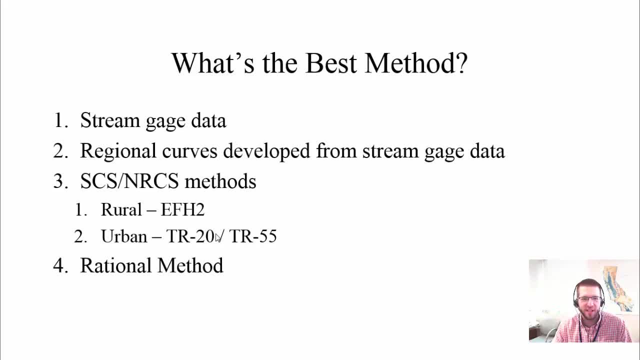 OK, so you can't use them on your one acre watershed leading to your catch basin- OK. next best is something is how we get into hydrologic models- OK. next best is something is how we get into hydrologic models- OK. next best is something is how we get into hydrologic models. 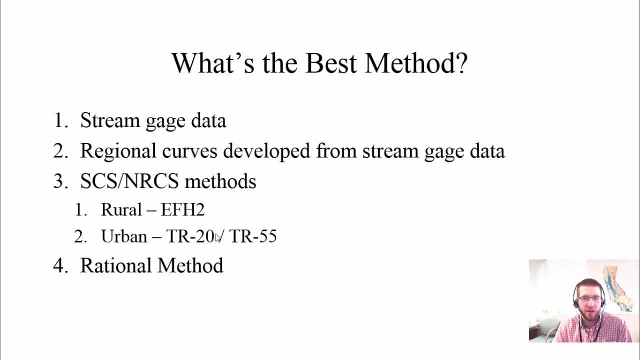 OK, so the Scs. it formaly called Scs, now it's called NRCS. OK, so the Scs. it formaly called Scs, now it's called NRCS. They have two methods For rural sites. you can use EFH 2.. 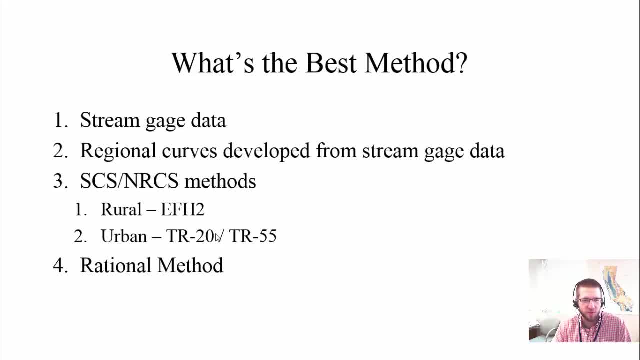 For urban sites, you can use TR 20.. Which is sometimes called TR 55,, which is the pen and paper version of the TR 20 method, TR 25, which is the pen and paper version of the TR 20 method, And then, finally, I say the least reliable is the Rational Method. 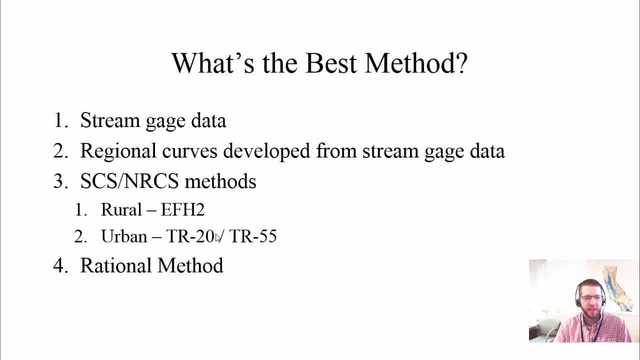 And then, finally, I say the least reliable is the Rational Method, And for that it is fine. So let's talk a little bit about where you would learn more about each of these topics, because we're not going to cover them all in this course. 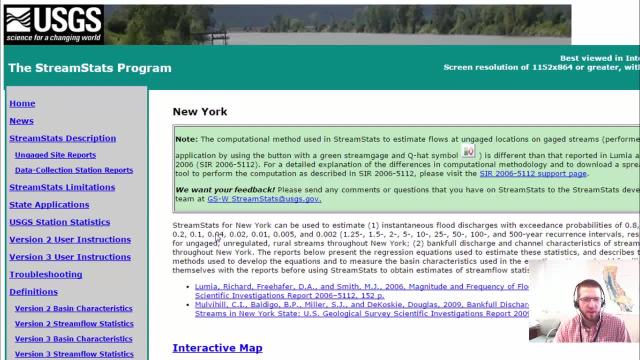 Okay, for stream gauge data and regression curves you need to go to your state's stream stats program. For New York it looks like this And each stream stats program has background documentation. For New York it's these two documents, Lumia and Freehofer, is magnitude of frequency of floods in New York. 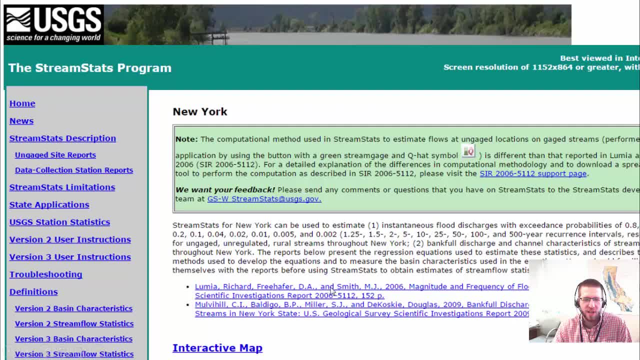 That covers drainage area and peak flow, I believe, And then this one covers bankfull discharge and channel characteristics. So for New York we have two components of stream stats: one for the bankfull channel cross-section and one for the magnitude of frequency floods. 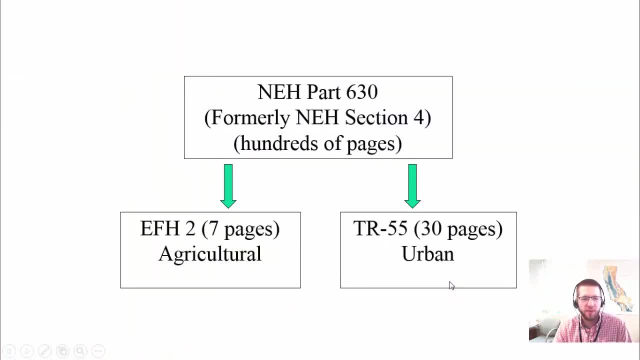 All right, how about TR55? Any opinions? And EFH2, those are both derived from the National Engineering Handbook, Part 630.. Okay, it used to be called NEH, Section 4. It's an NRCS publication. It's hundreds and hundreds of pages. 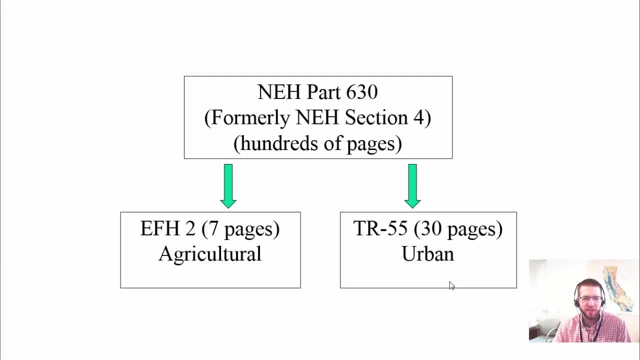 You do not want to read it, But there's two derived documents that are worth reading. EFH2 for agricultural lands. It's only seven pages. Download it from the NRCS website Or I've attached it here as an attachment to this lecture. 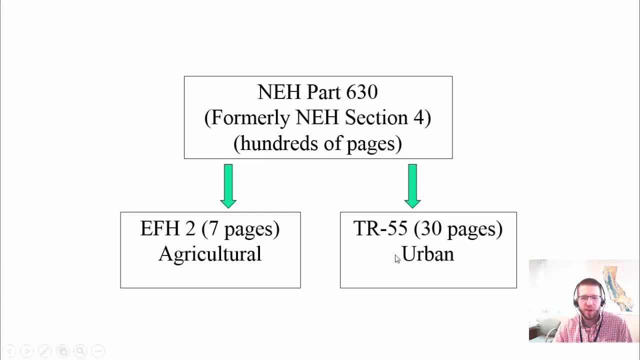 TR55 is also a good resource. Like I said, it's kind of the pen and paper version of the TR20 method and the TR20 manual isn't really helpful because it's a software program, but the TR55 manual is really helpful. 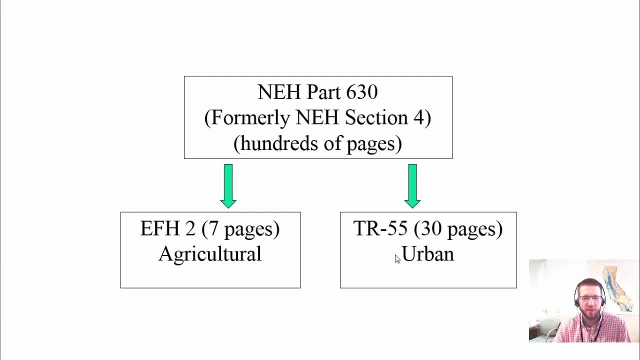 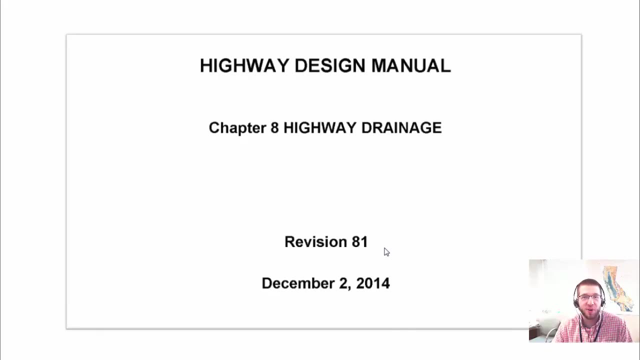 It goes through the steps and how each equation is derived and how to use it, And I've also attached this to this lecture. The only place I found it online is the HydroCAD website. I'm not really sure why. that is Okay and the Rational method. since we're in New York State, I'm going to recommend the New York State DOT Highway Drainage Manual or Highway Design Manual, Chapter 8, Highway Drainage. 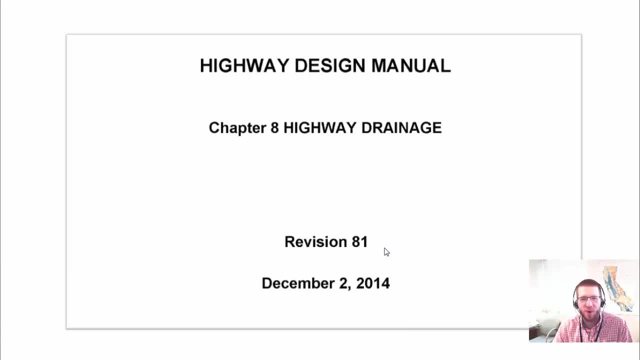 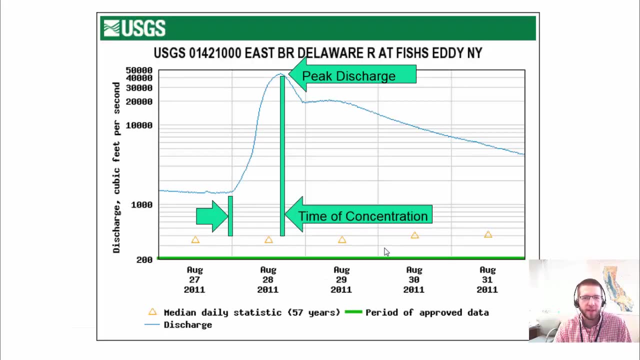 Okay, it has a nice little section on the Rational method and kind of where it came from and how to use it, But we will be covering the Rational method in this series. So I mentioned hydrographs before And you might be asking: what is a hydrograph? 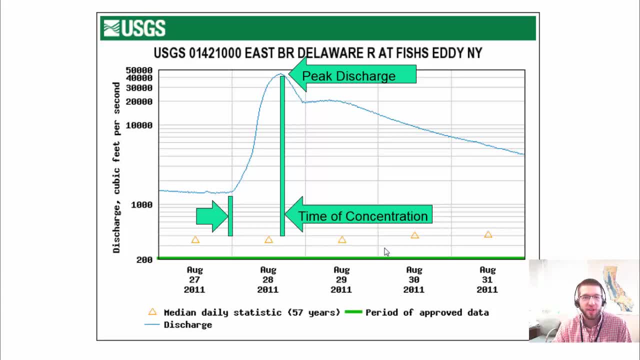 Well, it just shows the flow rate in a stream Over time. okay, in our cases, we're going to be developing hydrographs for a set amount of time, typically a design storm length, But this is just a regular one for a river. 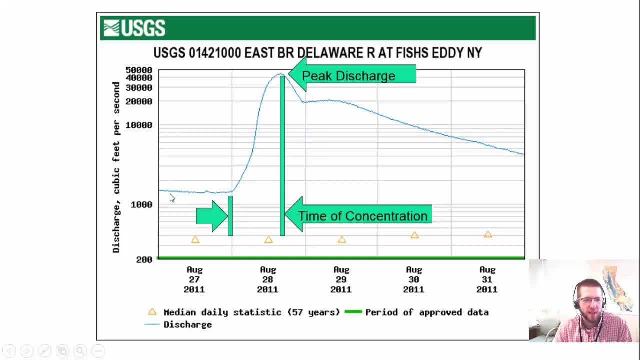 It's East Branch, Delaware River after Hurricane Irene. You can see, you know, before the flows reached the gauge, it was- you know this level- just over 1000 CFS. And then, once all the water in the watershed got down to this gauge, it was just over 1000 CFS. 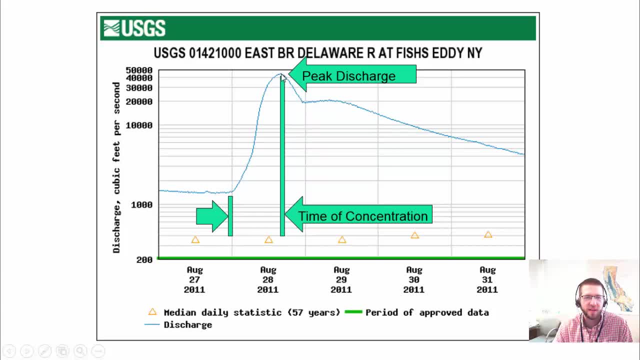 And then, once all the water in the watershed got down to this gauge, it was just over 1000 CFS. And then, once all the water in the watershed got down to this gauge, it was just over 1000 CFS. And then, once all the water in the watershed got down to this gauge, it reached a peak. 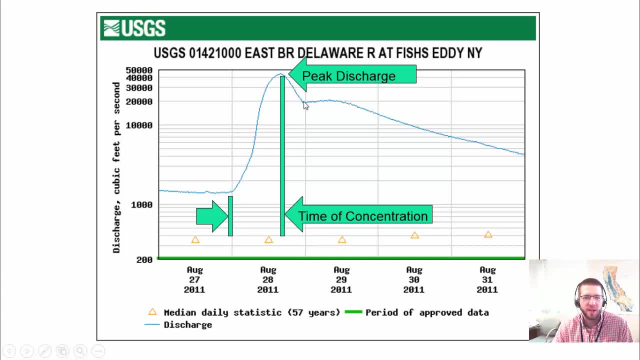 And then, you know, after the storm was over, it kind of gradually settled down. They had some flood control measures, which is why this is level, And then they let more water out and, you know, gradually went down. So this is kind of what we're looking at when we think of a hydrograph. 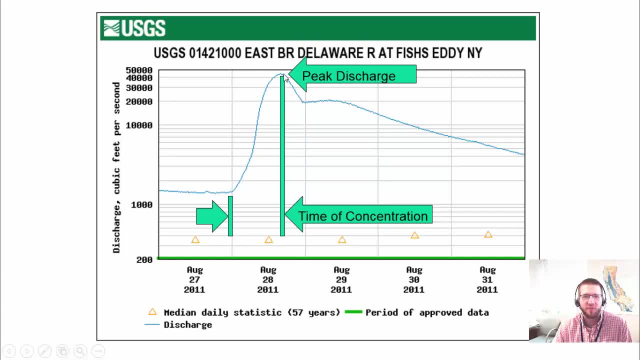 This top is just the peak discharge And a lot of our practices. we only need the peak discharge, This time window from when the flow at the design point or the gauge when it starts increasing to the peak discharge. that's called the time of concentration. 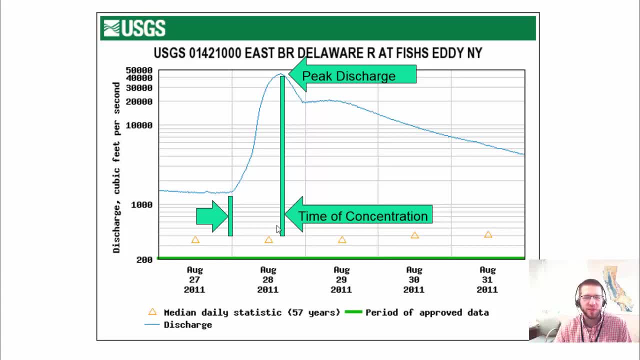 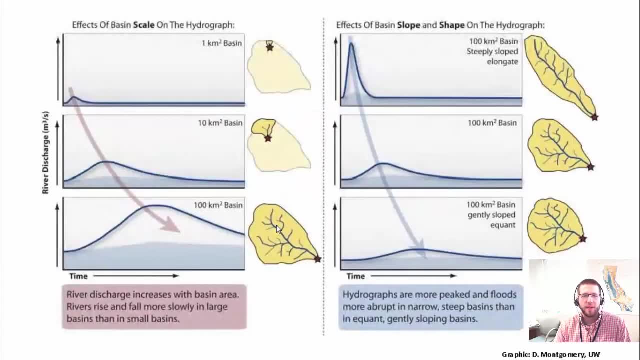 That's the time that it takes the furthest raindrops in the watershed to flow all the way down to the design point. Now, different watersheds are going to have hydrographs with different shapes, And I'm going to cover that in this slide. 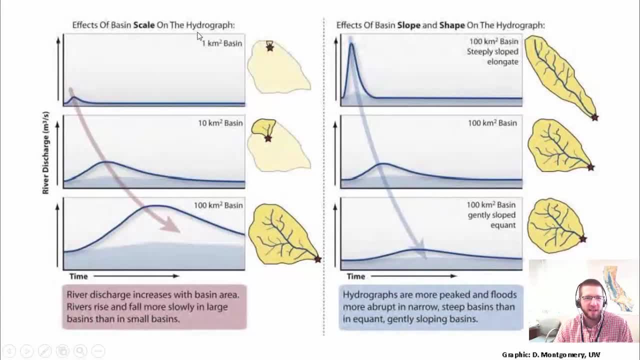 On this side it shows the effective basin size on the hydrograph. So very small A watershed. well, I wouldn't say. this is small, one kilometer squared. but you know it's a small peak flow with a short time of concentration. 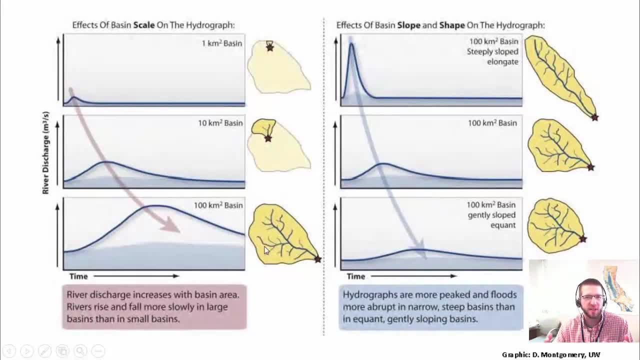 As the basin size gets bigger, obviously the peak is going to get bigger, but also the time of concentration will increase as well, right? So in this first one it only takes a short time for the furthest drops to get to the design point. 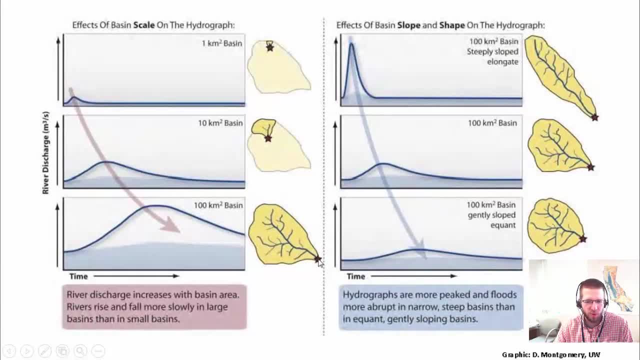 In this one it takes much longer for the furthest drops to get to the design point. OK, And basin slope and shape is going to make a difference too. OK, If you have a basin that's steeply sloped and elongated, you'll have a short time of concentration with a high peak. 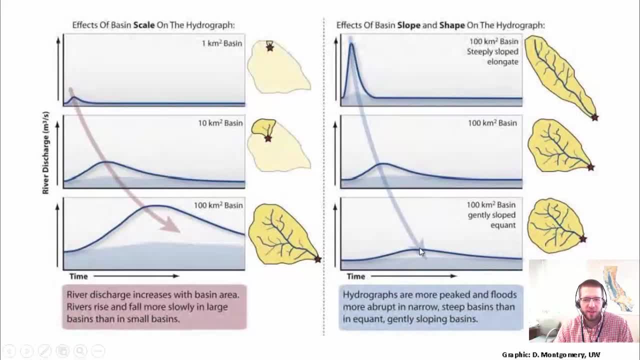 The more diffuse it is and flatter, you'll get a lower peak discharge and a longer time of concentration. I think in this — for these three examples, they're all the same area, say in square kilometers, color, But plus the Embraer difference. we should think about it. we should think about the rapid application. 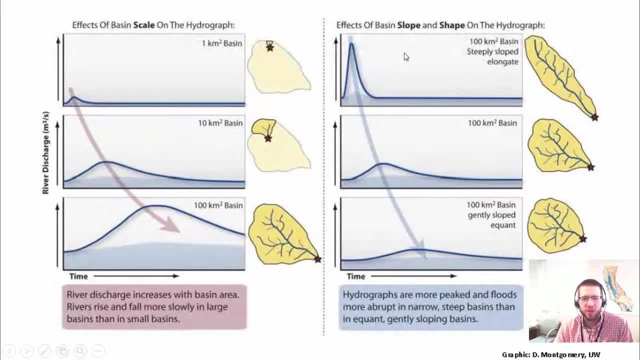 In the clear vagy regen the새 in чер. In the later phase of- hopefully until the end of these technical world events. they make up a bigger difference than that. They're each going to have a different time of concentration and peak flow. 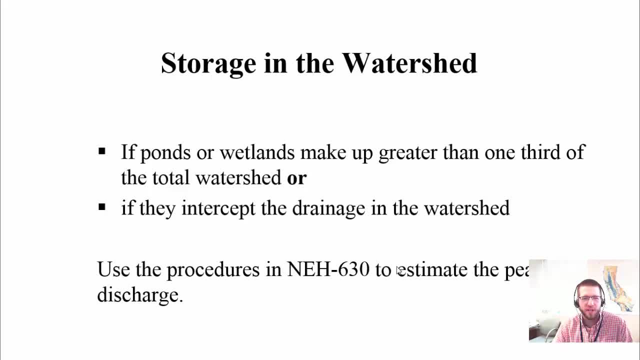 Now, one thing to consider is storage in the watershed. If there's ponds or wetlands in your watershed, you need to take those into account, because water in your watershed will collect in those areas instead of just flowing straight down to your design point, And you can use NEH 630 to estimate the peak discharge in watersheds- in rural watersheds, I would say. 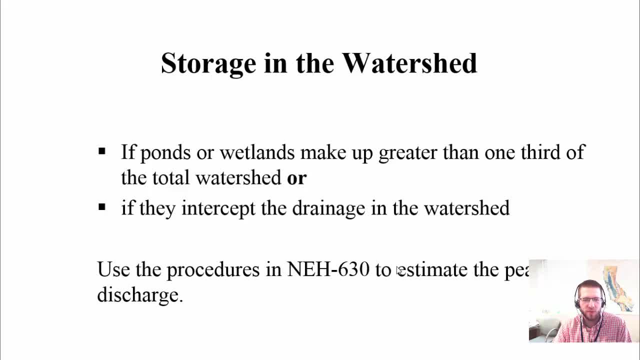 In urban watersheds with storage you should break it up into sub-watersheds and use a modeling program such as HydroCAD to figure that out. But I think for rural sites you can use NEH 630.. They have adjustment factors for ponds and wetlands to help you figure out what the modified discharge would be for those. 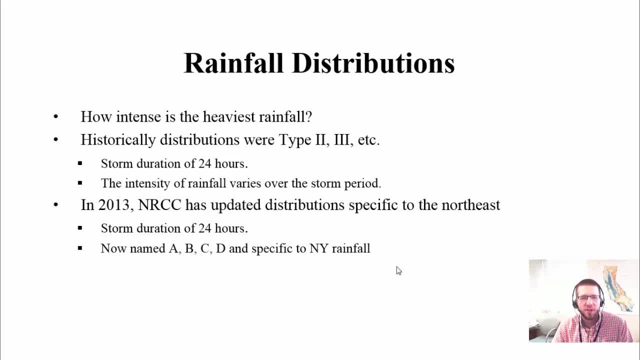 Now I want to talk about rainfall distributions. We're trying to come up with how much runoff runs off a site, So we need to know, kind of, how much rainfall hits the site And we want to know how intense is the heaviest rainfall, because that'll produce the greatest flow rates for our BMPs. 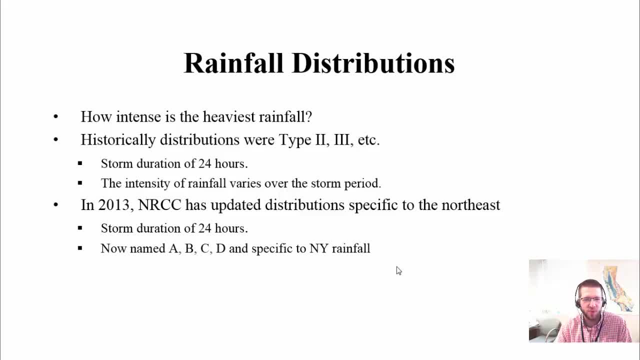 Historically we had synthetic rainfall distributions called Type 2,, Type 3, etc. It was a storm duration of 24 hours and the intensity of the rainfall varies over the storm period. In 2013,, the Northeast Regional Climate Center updated rainfall distributions for the Northeast United States and New York Falls in that. 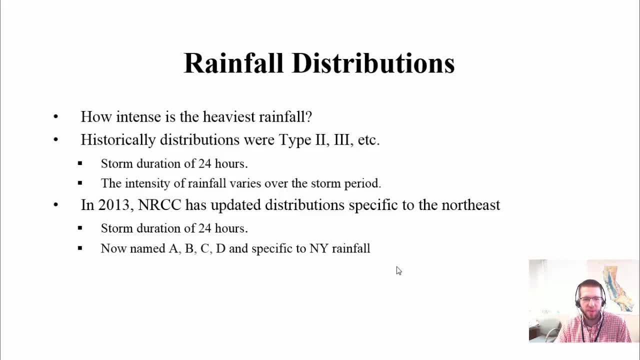 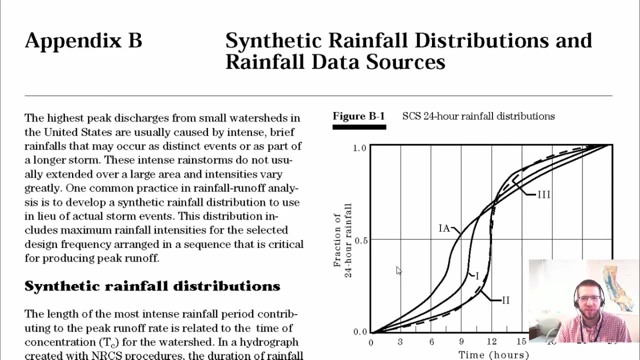 So we should be using the new rainfall distributions Type A, B, C and D, And these are also 24-hour storms. You might be asking: what is a synthetic rainfall distribution? Why do we use it? Well, I'm not going to explain that right now, but I want you to go to TR 55 at Appendix B and read the sheet on synthetic rainfall distributions. 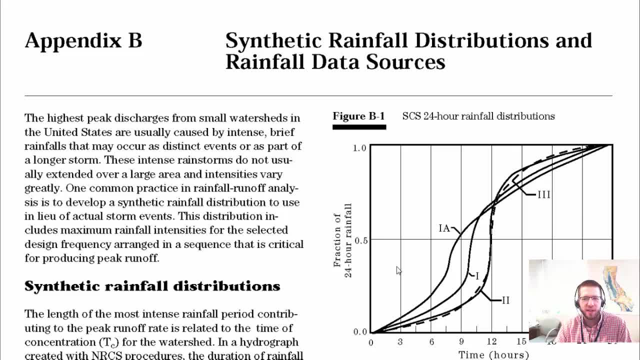 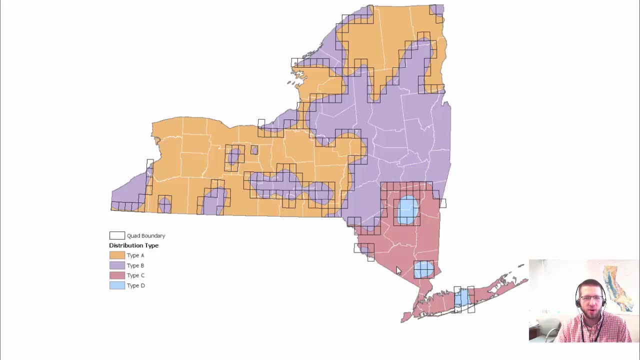 It's actually a pretty handy tool for doing hydrology so that everybody can be using a uniform format of data. We can get individual rainfall amounts, but we're coming up with intensities that are kind of uniform across the field. So if you're looking for the synthetic distribution type in New York, you can go to this map on the NRCS engineering website for New York. 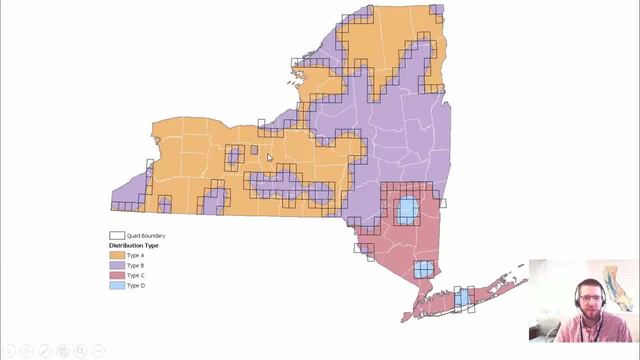 And it just has all the counties and it says whether you're A, B, C or D. Okay, if you're on one of these tiles that is a border between two of the types, there's blow-up maps of those and it'll show which towns are in which types. 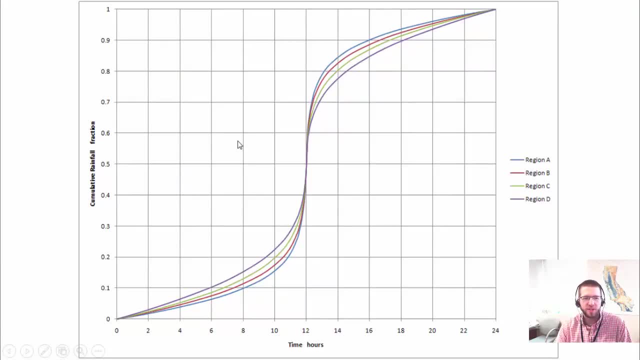 And then, finally, I want to show you this map. This is a map of New York. This is a map of New York And I want to just show you the distributions. This is what it looks like. This is a synthetic rainfall distribution curve.